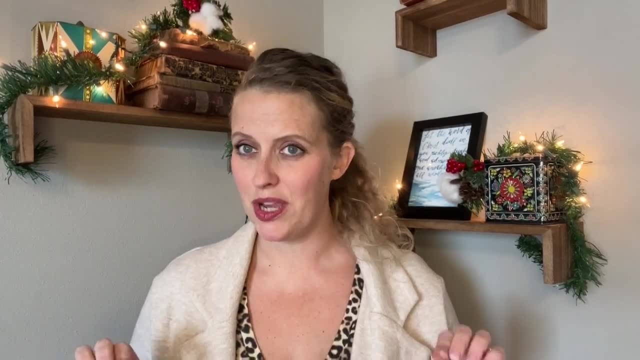 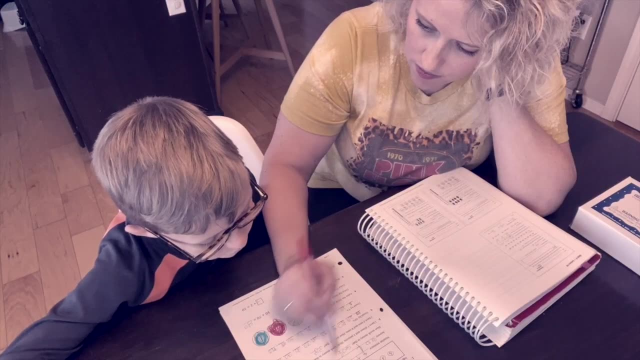 Okay, guys, I really think I found like a hidden gem of a math curriculum for preschool. Let's talk about it. If you're new here, I'm Ryan, a Christ-following wife and homeschool mom to three boys. Here we talk all things homeschool and we will learn together how to use our roles as wife. 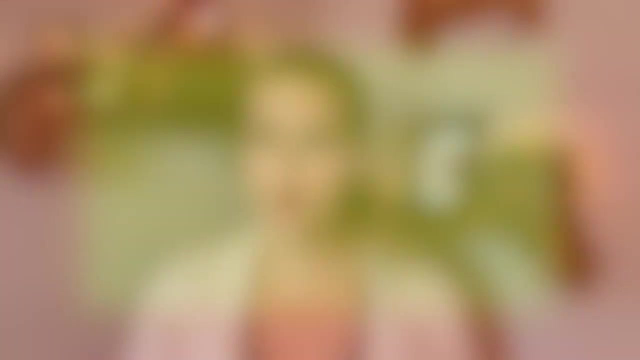 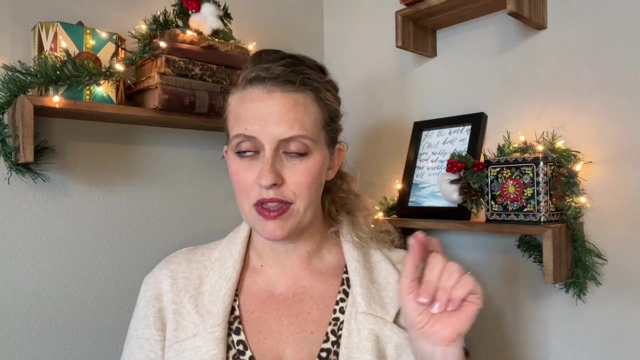 mom, teacher and homemaker in order to glorify God. For me preschool math I've gone back and forth. I've used just the regular workbook, where you know here are three fish and you write the number three and then there's a plus sign and then there's two more fish and you write the number two. 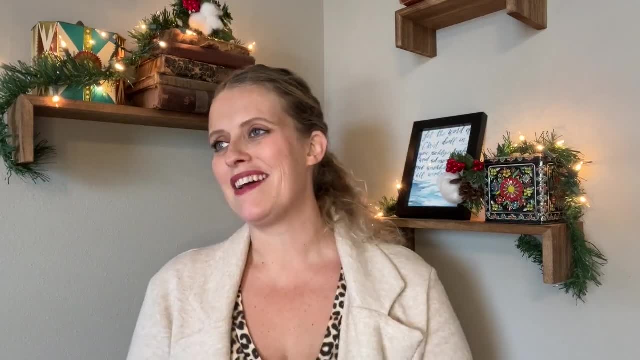 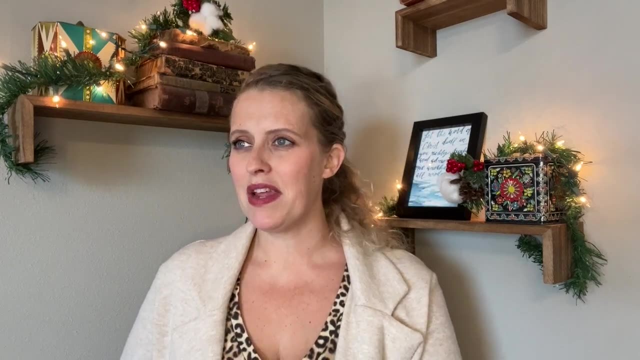 and then there's a picture of five fish and you write the number five, right, And that's kind of stuff I remember doing when I was a kid and I think that stuff has its place and is well and good. But I think math needs to be a little more hands-on, for younger kids especially, And so then 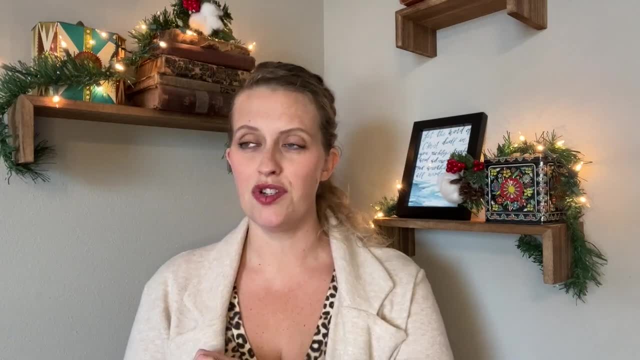 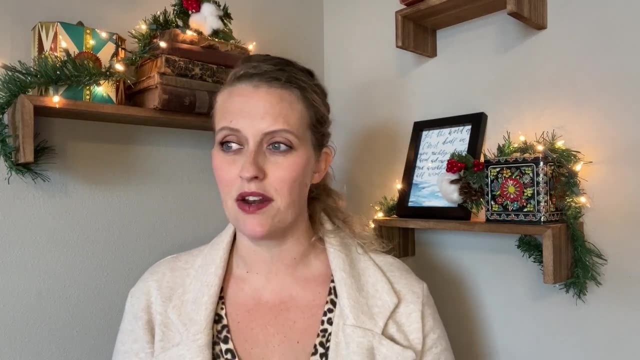 I've also done the complete opposite, where I've done just play with these manipulatives and here show me three teddy bears, and they show you the three teddy bears and you take one away and all the things, And I think that's good too. But I was looking for something kind of in between. 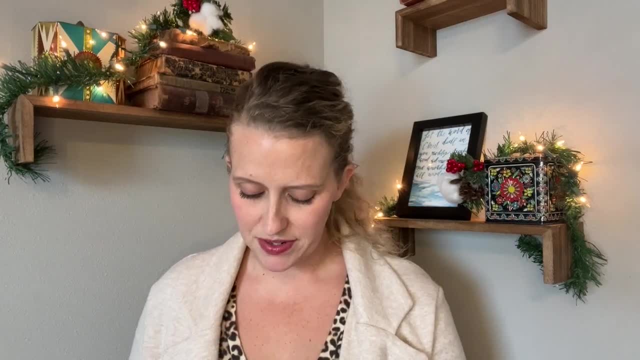 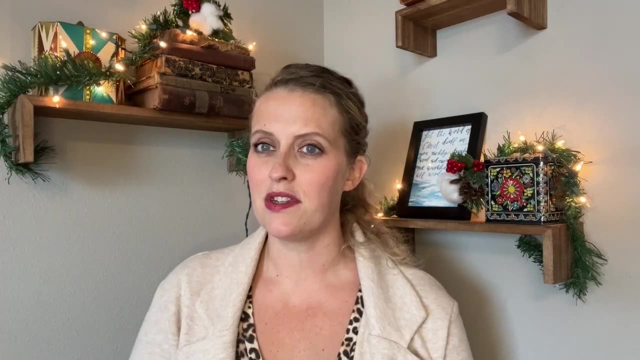 and I think I've actually found that, And what we're going to talk about today is mathematical reasoning and this is by the Critical Thinking Company, And this is something that I just was looking around YouTube one day saw that someone was using it. I'm like: what's that? And I looked 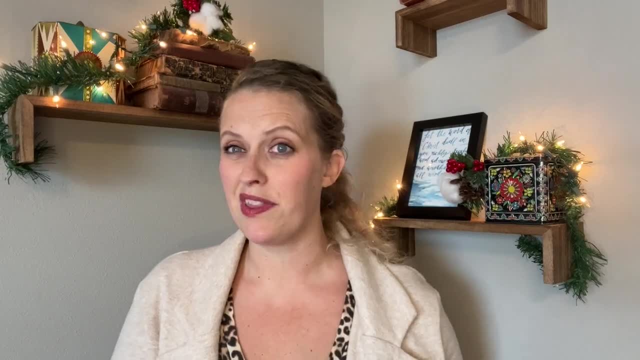 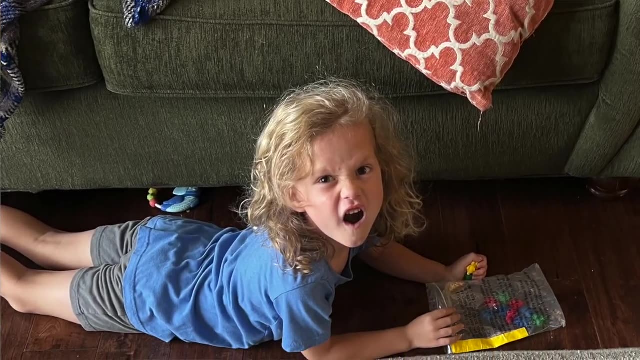 into it. I have not looked at their older grades, so if you have any questions about that, I am not the one to ask. But I picked this up for my four-year-old At the beginning of this school year and so far we are loving it. We did go ahead and get two books. 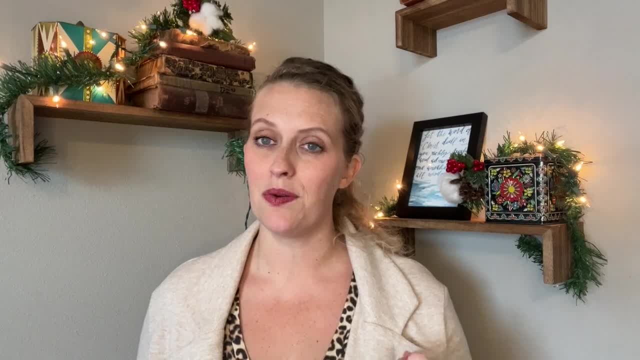 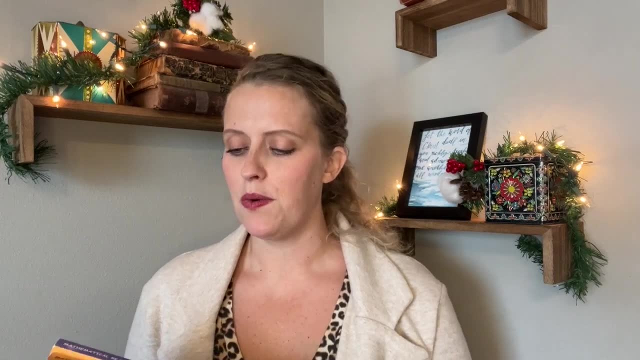 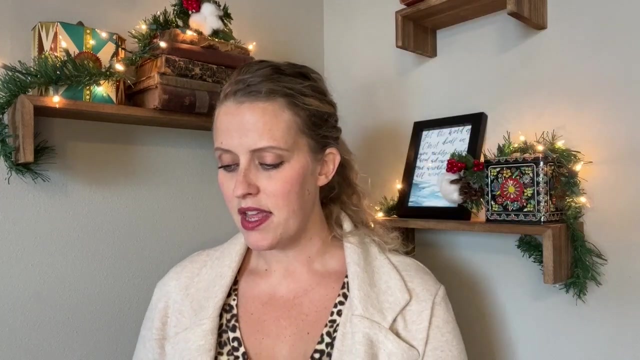 because one they were at our local homeschool shop for next to nothing and they were not written in and both of them were there, So I just picked them both up. But also, my son was four at the beginning of the school year. He won't turn five until next semester. But these books, the first 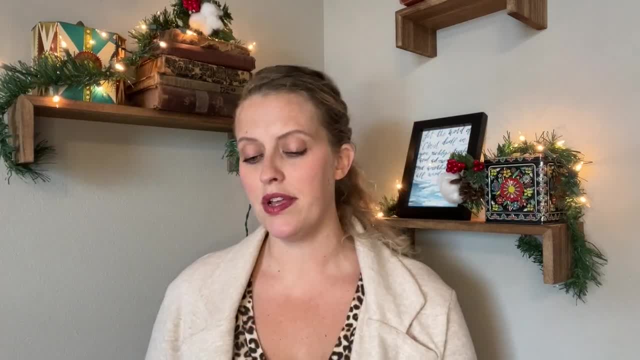 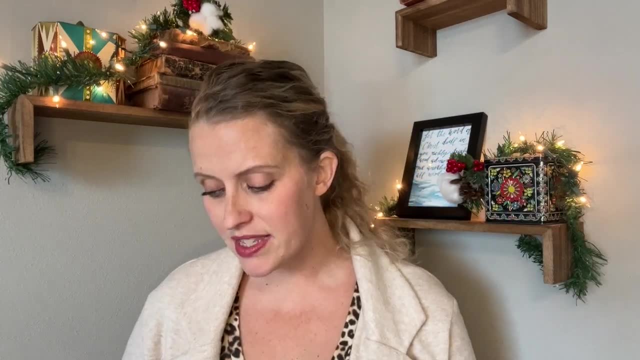 one is meant for age three and then the second book is meant for age four, So really this should have been what he went through this semester. So I'm going to go ahead and get two books, And this is going to be the first book that I'm going to talk about this whole school year. 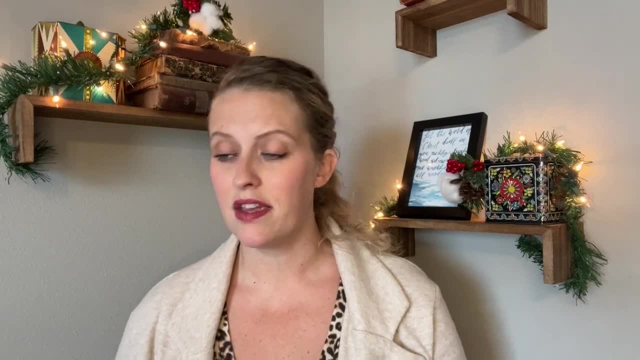 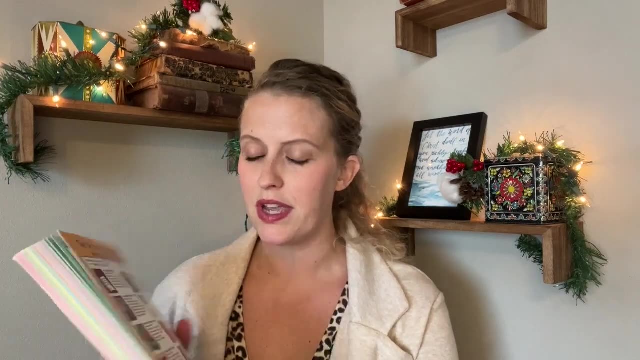 However, because this approach is quite different from anything that he's ever done before, I wanted to go ahead and let him do the one for age three, And we've flown through it really fast. So we are almost done with this and we're not to semester yet, So I think we can easily finish both of these. 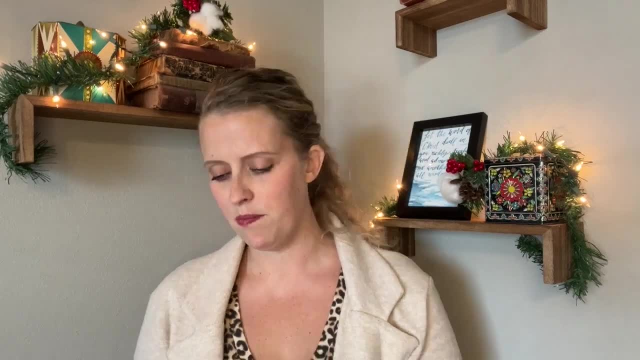 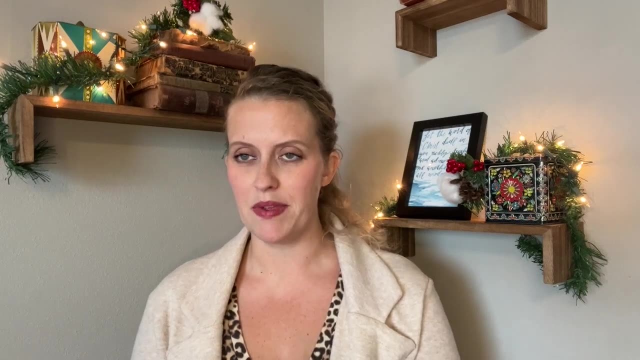 at least by the end of next summer, before we start his kindergarten curriculum, But chances are we will probably get done even before that. So this is going to look a lot different than anything you typically do before and you don't get to pick it up. This book is going to be a really fun book. 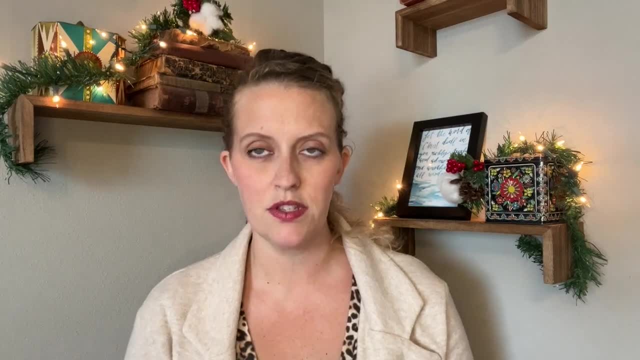 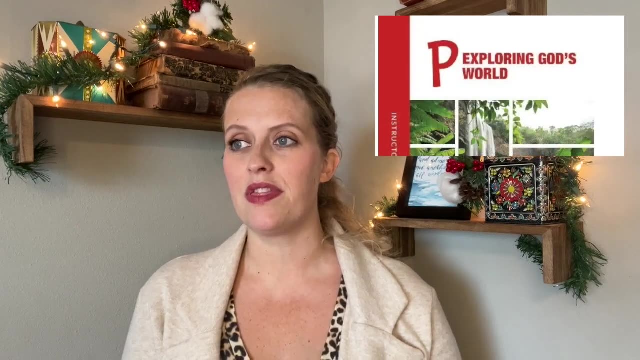 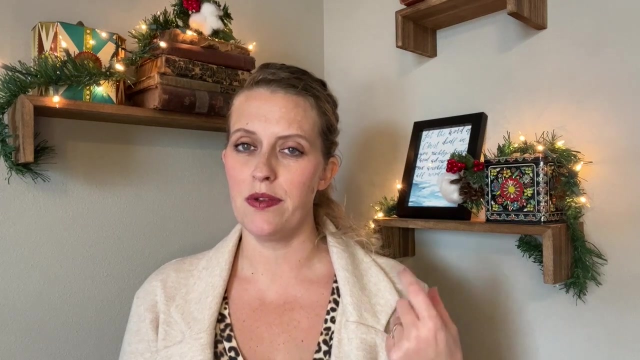 see in a math curriculum. So just for reference, we use Sunlight for his core, for his pre-K, and with that they work a lot on recognizing numbers. and we've started to work on, you know, using a. I forget what they call it, it's like a tens block, but it's not a block anyway. 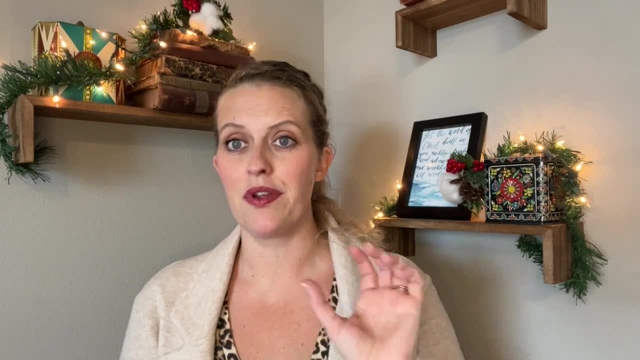 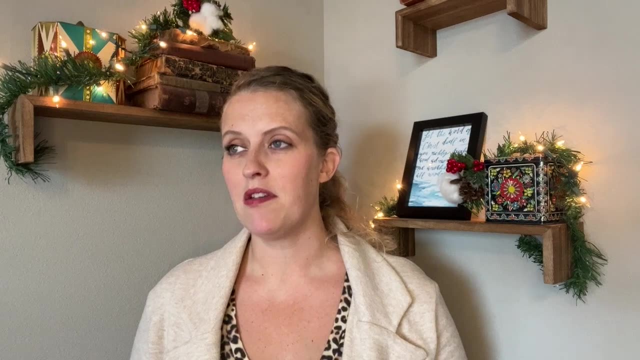 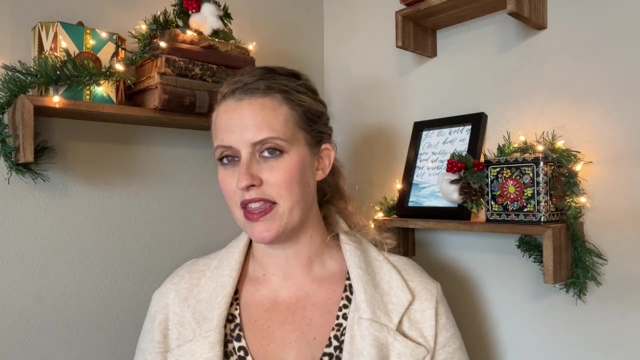 but like seeing tens versus 100s versus singles, right, So we started working a little bit on that. but it's a lot of number recognition and counting, pretty basic stuff. They don't go very much into math. so I wanted something else to go along with this, and so when I found this, I was 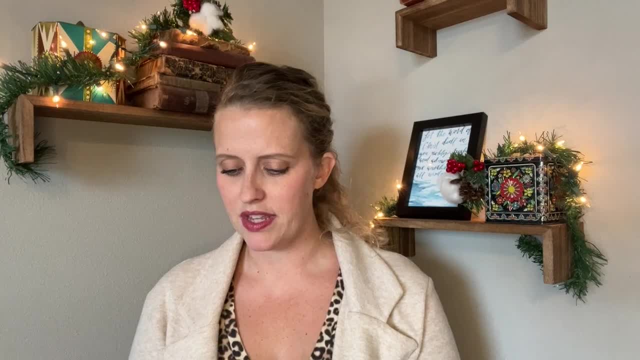 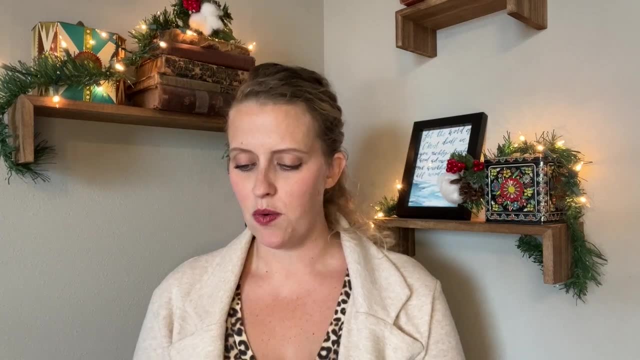 like I think this is what I want. So there is very minimal handwriting in this. This is a lot of tell me point. look at touch, blah, blah, blah, blah blah. So when you're very first beginnings. 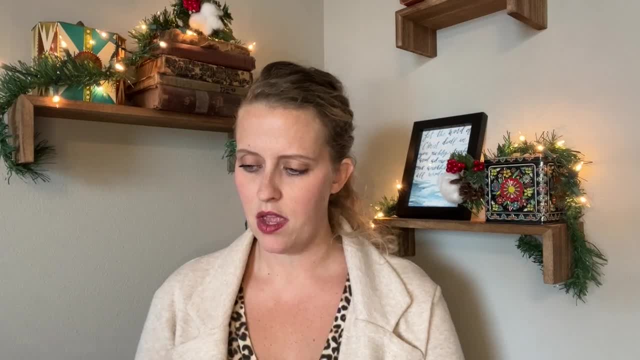 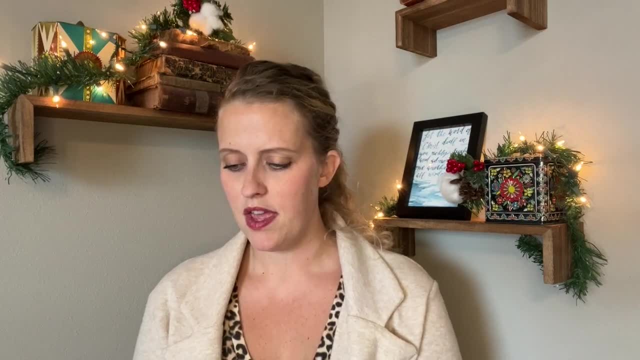 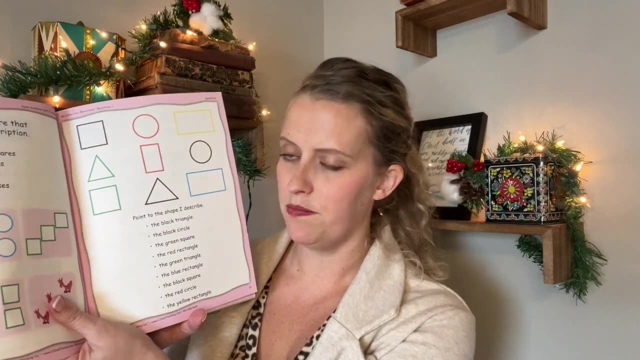 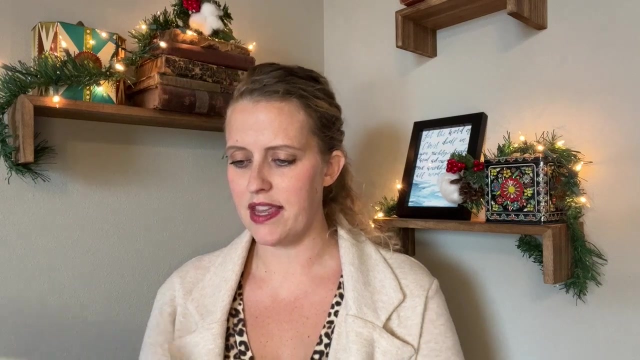 you count the objects, very basic stuff. And then there's also pages like this where it's like find the black triangle, So they have to find the color and the shape. Then there are things like this: how many caps are there? color three of them. how many circles, color three of them? 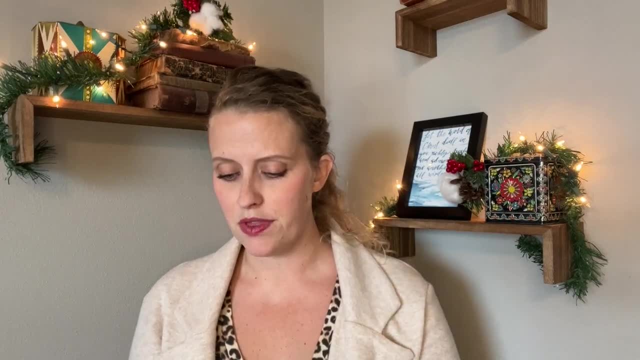 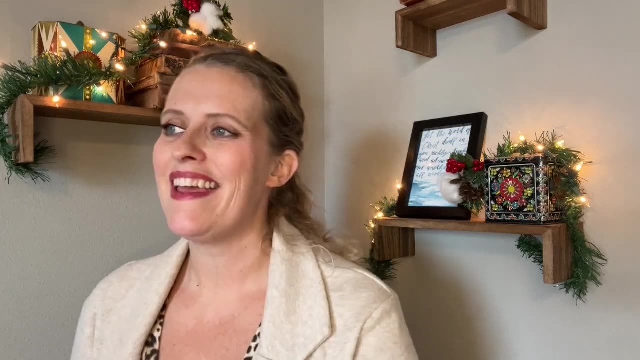 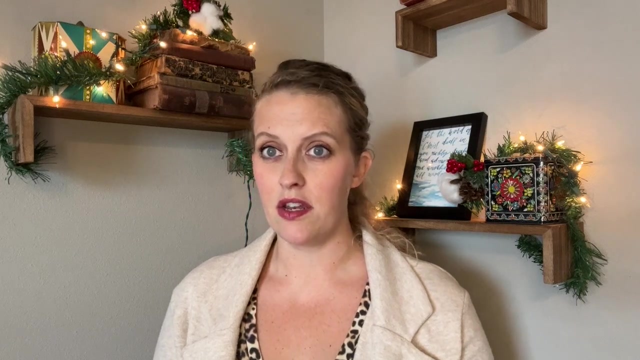 So it's listening to verbal commands and then following through with those. So this is a lot of. you know it's called math, Mathematical reasoning for a reason. It is not just adding, subtracting- Yes, they do touch on that, but it's a lot of. look, listen, obey, right, So it's a lot of. what is my mom telling me Now? 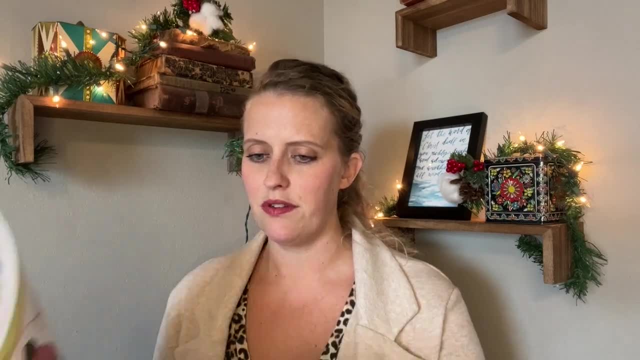 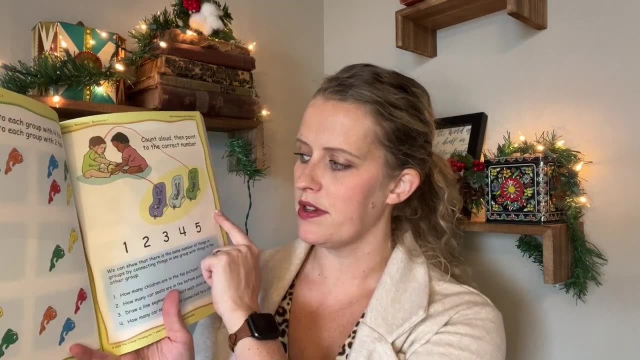 let me look at that and now let me do it. So here's another example: point to each group with four fish, point to the ones with two fish. This one, count out loud and put each baby with a car seat. How many car seats you have left over? That kind of thing They really focus on in this younger 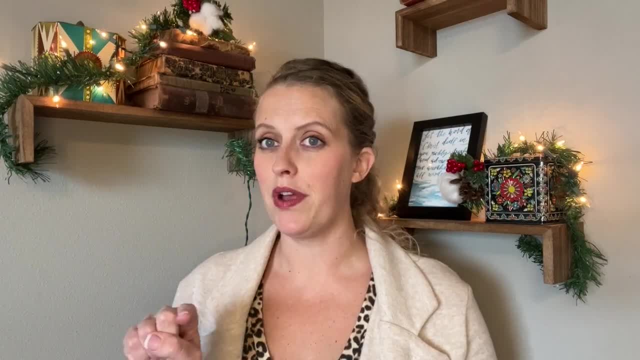 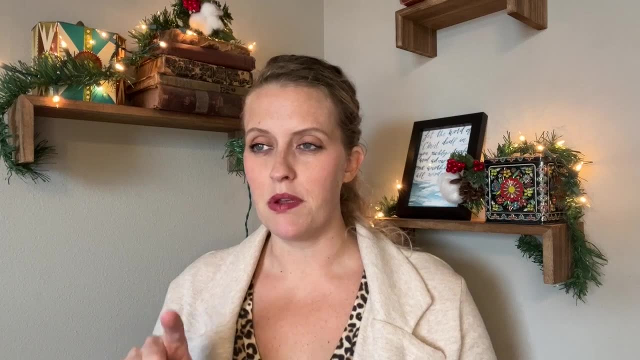 grade, wanting you to be able to look at a picture and, without counting one by one, know how many are in there. you know, obviously like smaller numbers, but to be able to look at three ducks and not have to go one, two, three, but to look and go: oh, that's three ducks, right, They talk a lot about. 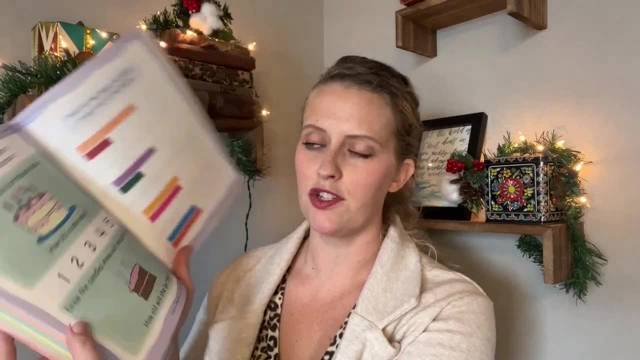 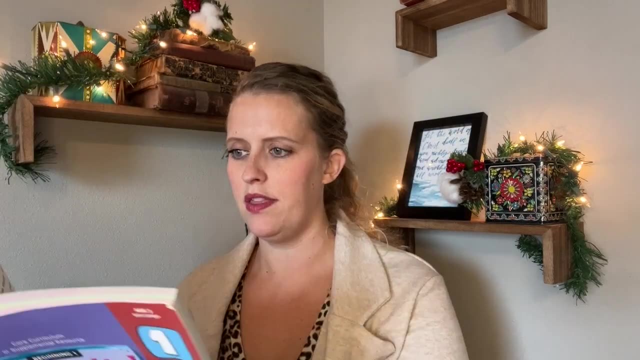 most fewest, longest, shortest. They talk about ordinal numbers and about you know, standing in line, who's first, who's second, who's third, and then stuff like this. Like this is data analysis. So which one of the two things would be faster, right? 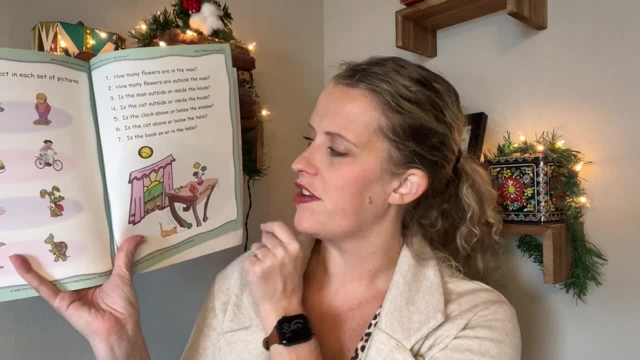 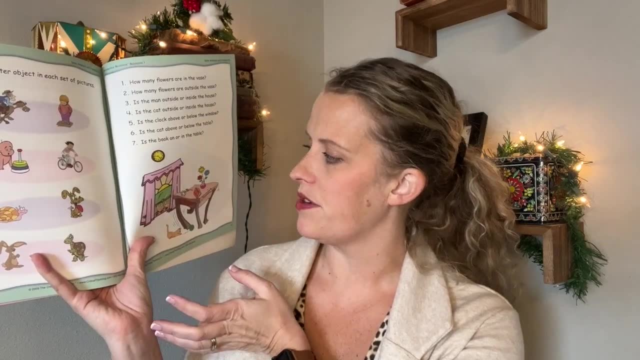 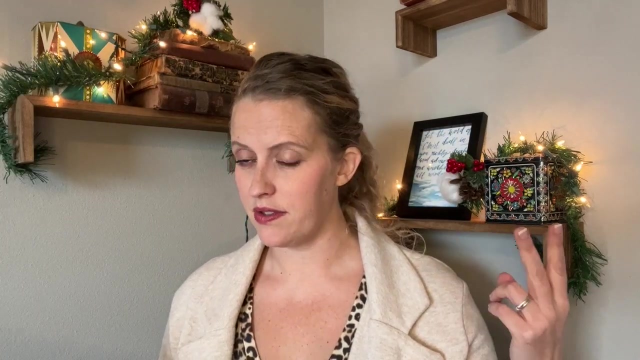 Um, this one. you see a whole picture, but then it asks you very specific questions: Is the book on or in the table? Is the cat outside or inside? How many flowers are there, Things like that. So, throughout the whole thing, they're working on counting, They're working on fractions. No, it sounds kind of weird, but how? 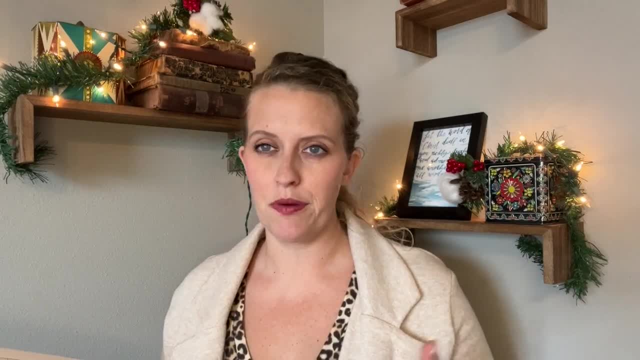 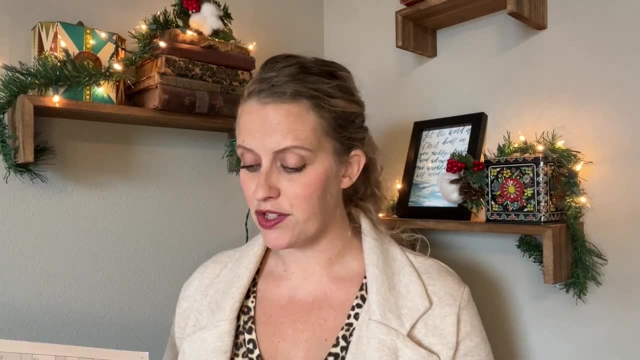 many out of the four people are wearing a blue shirt? Two out of four. Okay, So not fraction, fractions. Um, then there's work on language. So, again following those directions. um, manipulatives, there's matching, there's ordering, there's patterns, there's shapes. 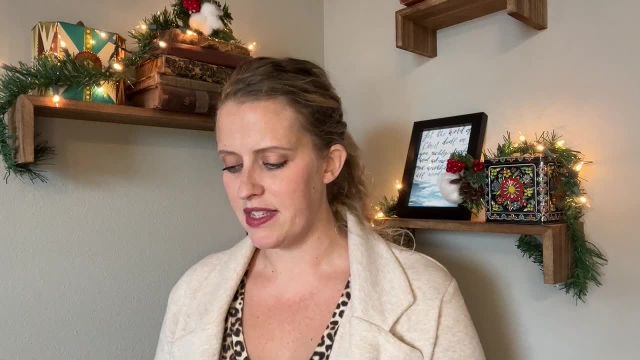 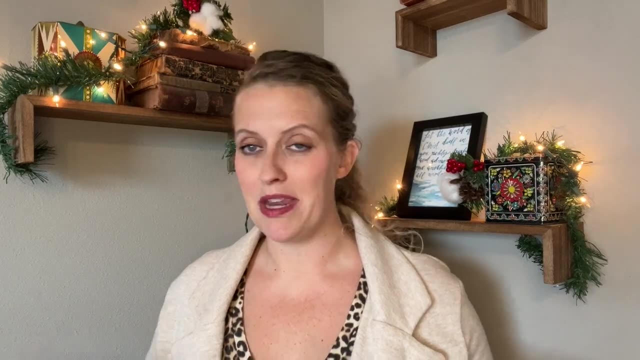 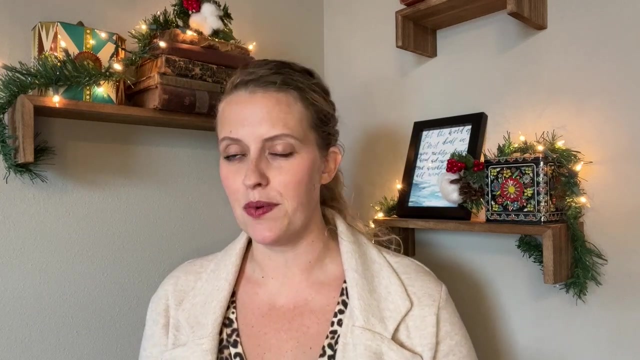 and subtraction. So it touches on a lot of the basics, but in a very I like it because it's tangible, but there's not a lot of little pieces right, I don't have to get out all the manipulatives Like it's all right here, but it's very much point and say, or trace this line or do. 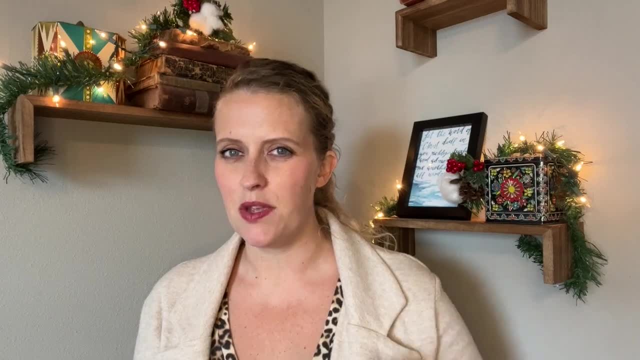 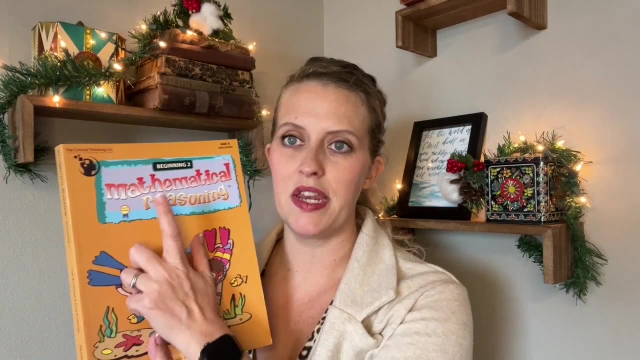 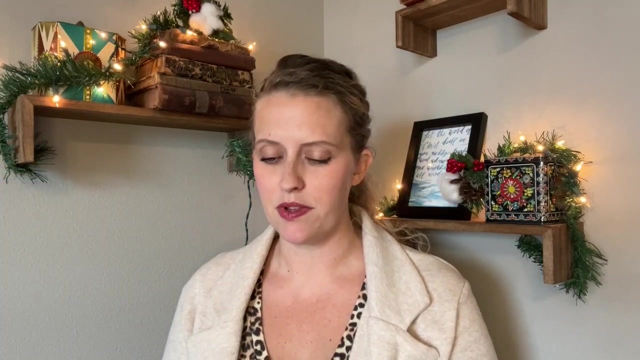 whatever. There's very little um, like busy work, handwriting type stuff. So that is for age three. this one is called beginning two of mathematical reasoning and this is for age four. So, like I said, we'll start this one right around semester. So again, we're going to match our. 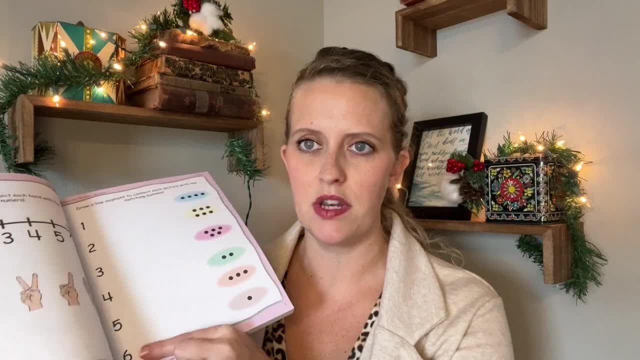 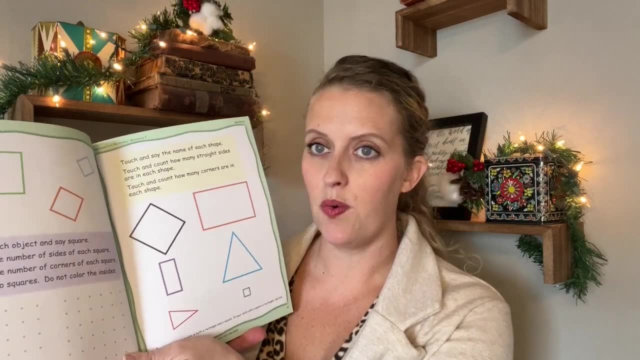 numbers, with the number of fingers. they're holding up the dots with the numbers. This is kind of number recognition type stuff. You're going to do some geometry So count the number of sides and the number of corners, and you're going to trace them or draw them. Then we get into actually. 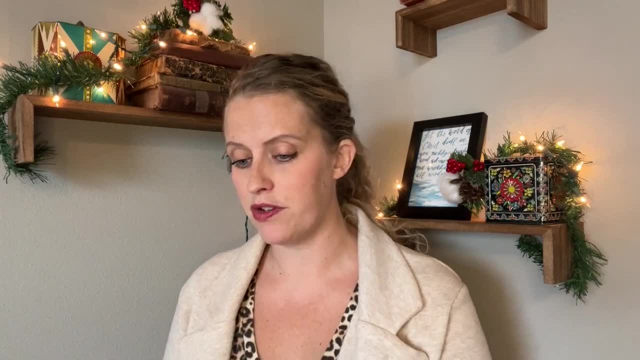 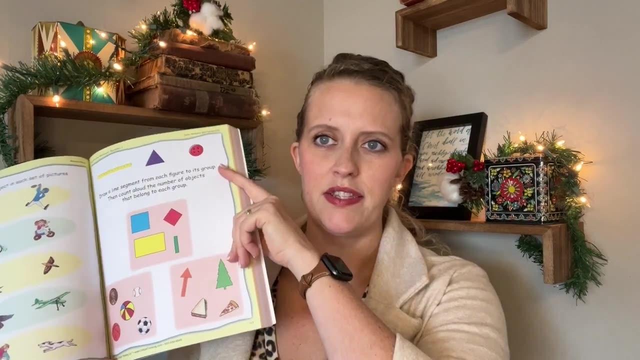 making our numbers, which sunlight works really heavily on writing your numbers earlier. So it's just kind of a reversal on how they choose to do things. And then this: we're putting things into groups. So these are things with different shapes and you have to draw a line to connect them to. 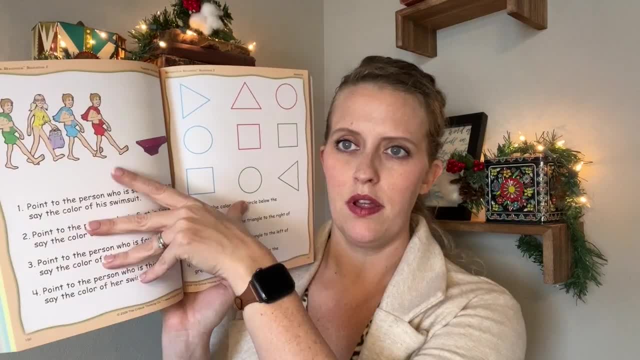 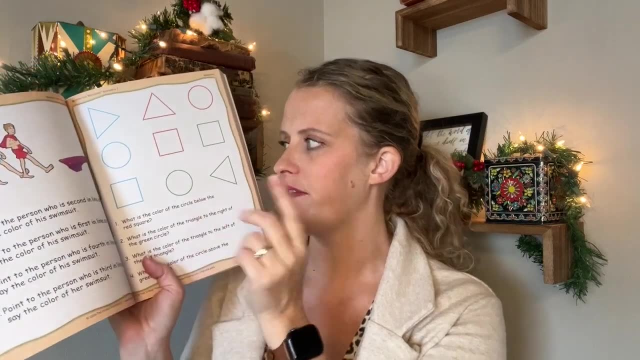 which group they belong in. Again, working on some more um ordering. and what is the color of the circle below the red square? So they have to find the red square. Then they have to think below, above, behind all those different things. 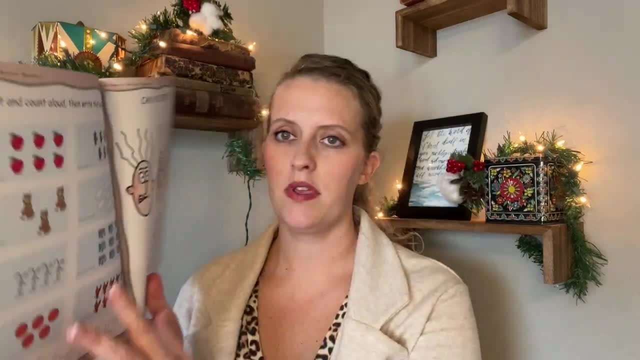 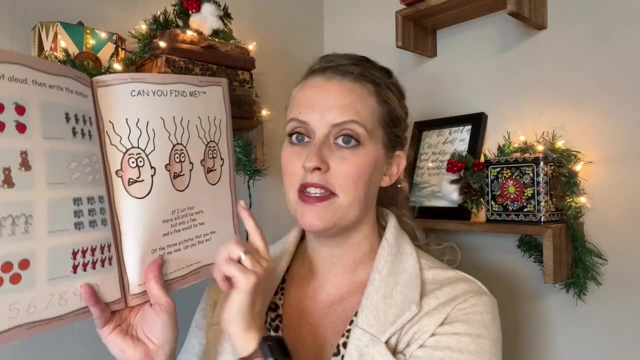 And then you're going to work on this. You're finding which thing does not belong in each set, Okay, And then toward the end of the year you would be actually writing the numbers on which things they go to. These were some of my son's favorite. I forgot to mention these in book three. 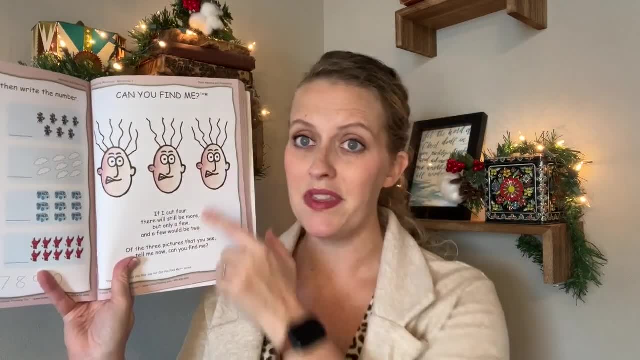 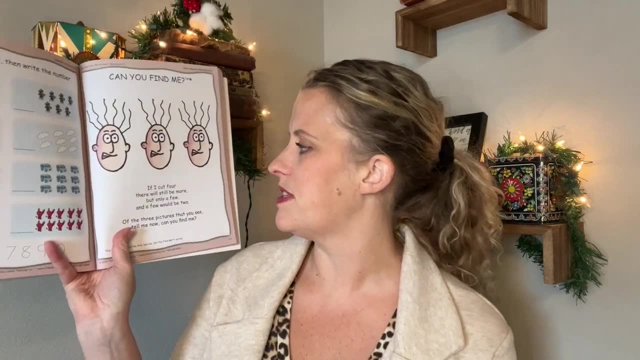 or age three book. So these are the- can you find me? And some of these are pretty tricky. So it's a little poem. You read the poem out loud and then to define which one the poem is talking about. So this one says: if I cut four, there will still be more, but only a few. And if you 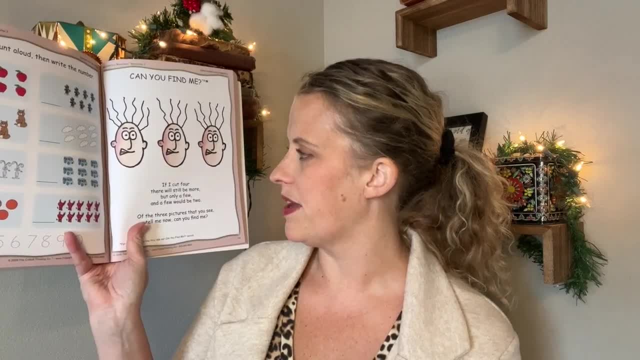 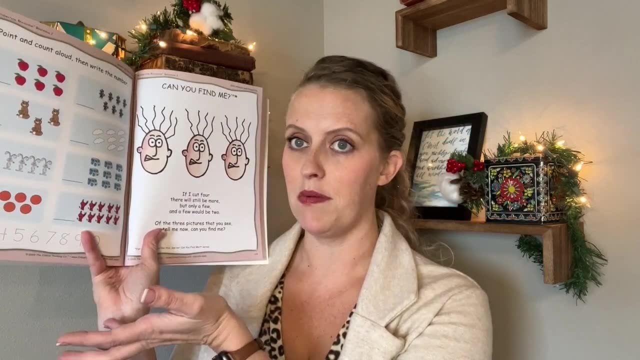 be two of the three pictures that you see. tell me now, can you find me? and so you're looking at his hair. so it's obviously not gonna be the one that has four hairs, because it says, if I cut four there would still be more. so it's not that guy. so is it this guy or this guy? well, this one has one, two. 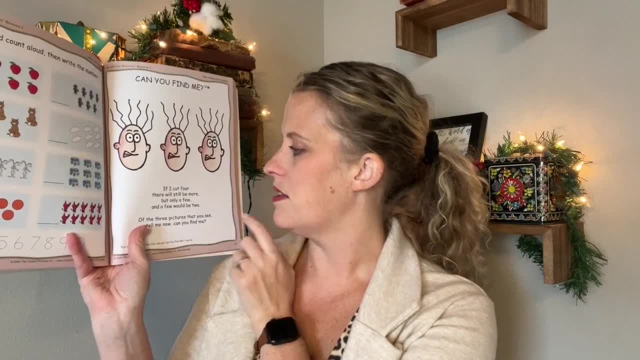 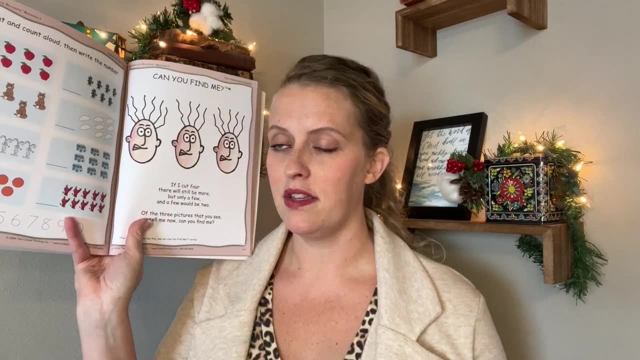 three, four, five, six. this one has five and it says: but only a few if you would be two. so if I cut four, there'd be two left. so instead of just saying okay, which one has enough hair that when you cut four there'd be two, they say it in a rhyme so that your kid really has to like sit and think about it. 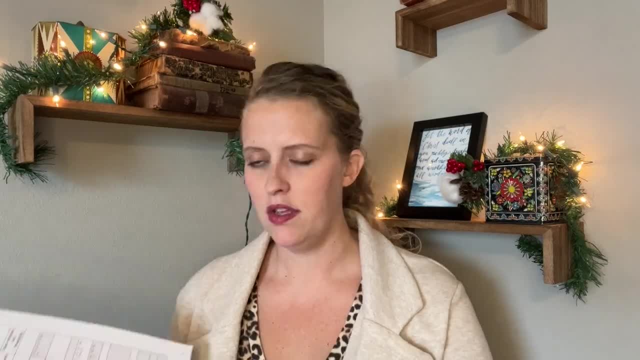 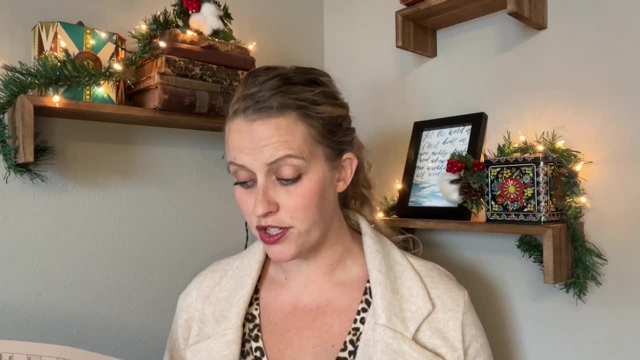 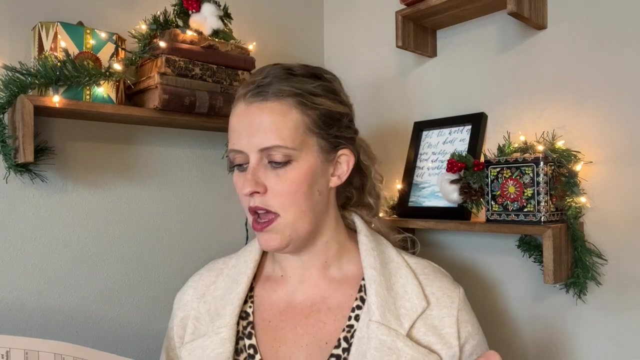 and my son did so well on those and they're really interesting to me. so this the scope and sequence. it's very similar: addition, application, counting fractions, language logic, manipulative, match, order, pattern, shape subtraction. so there's a little bit of differences in what they learn, but they're 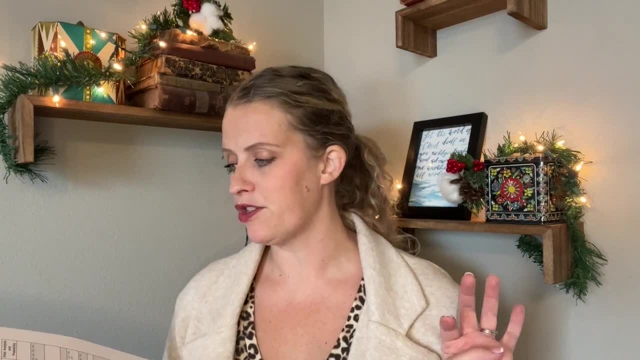 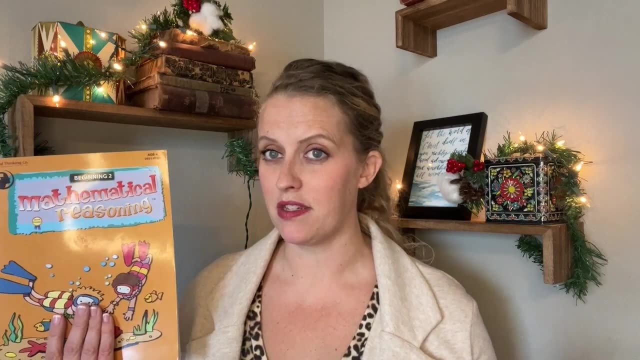 using number and operations using algebra, geometry, measurement, data analysis and probability: probability. so here's my pen and paper near case things that you just learned about the the math curriculum. so this is just laying the foundations for more logic-based learning as they get older, and that's. 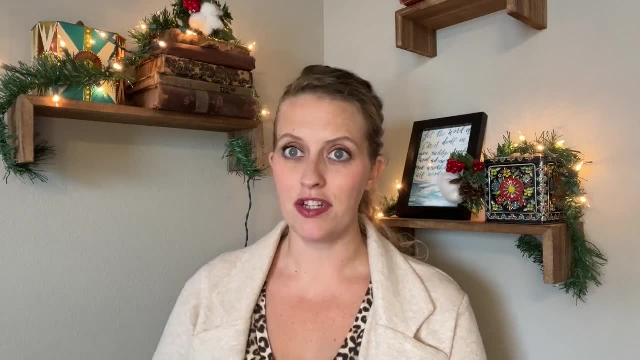 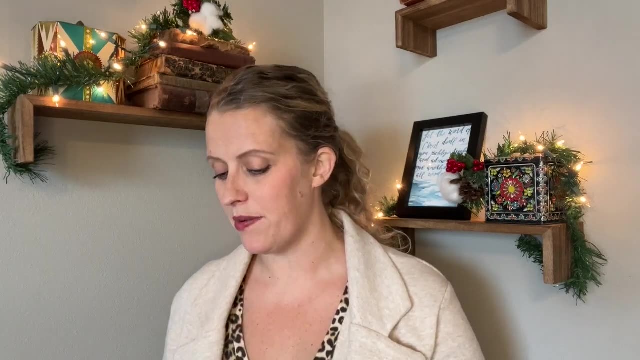 what I like about those little poems is that you really have to, you know, use deductive reasoning and logic to get that answer, so I am loving this so far. it is definitely not a traditional math curriculum, but it is something that I would definitely give a try if you are looking for. 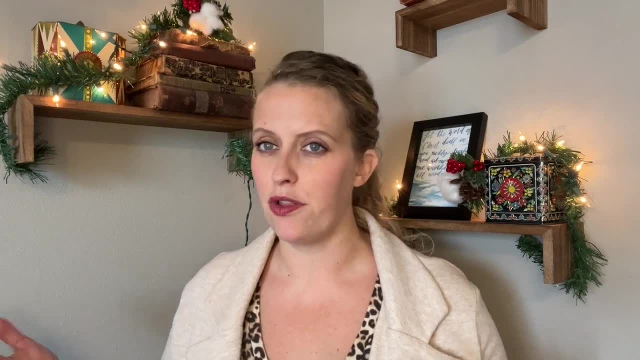 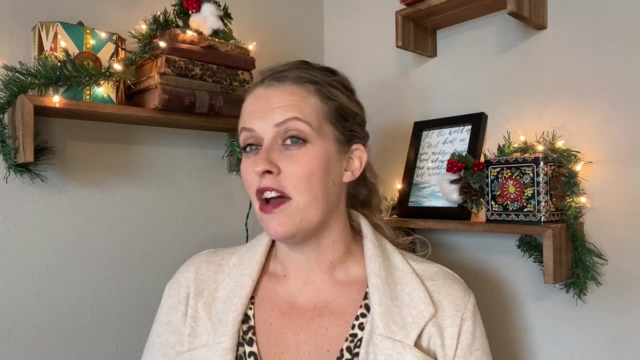 something that's not just your basic workbook and not just basic- oh, let them play and they'll learn how to do it- of both of those approaches- And I think this kind of meets in the middle. It is enough by itself, but I think it also could be very much a supplemental thing If you have something. 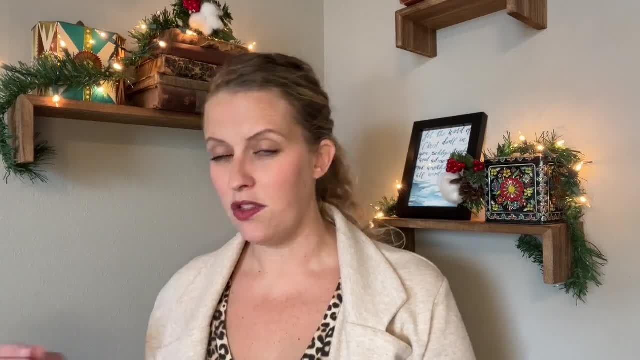 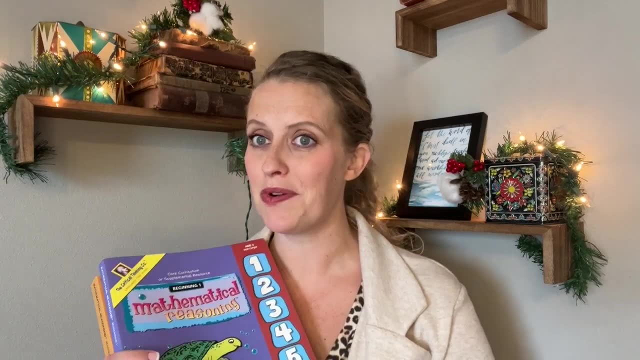 else that you're loving and using, but you're kind of wanting to get to that logic side of things in. I highly recommend this. So you guys had asked for this flip through. It was not super in-depth, but it's really just very point blank. You don't need anything else other than 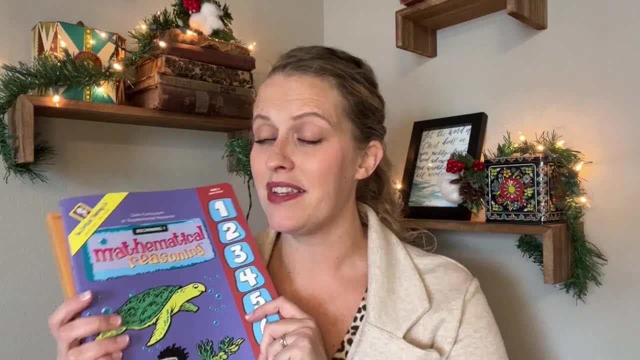 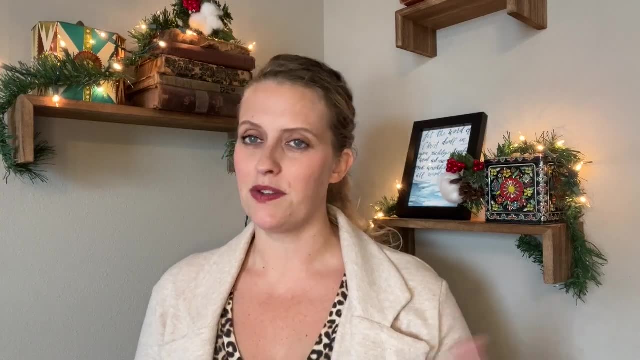 these books to teach it And I feel like my son has learned a lot. So, even though he's four and working through the age three thing, we're just kind of working through how to do this And, like I said, he's also getting the little bit of math that sunlight throws in there. So I'm hoping by